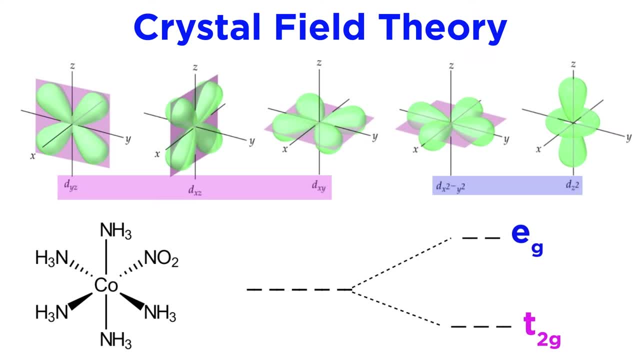 axes. So we introduced the concept of T2g orbitals, which are the lower energy dxy, dxz and dyz orbitals, and the higher energy eg orbitals, which are the dx squared minus y squared and dz squared orbitals, and we called the energy between them the crystal field splitting. 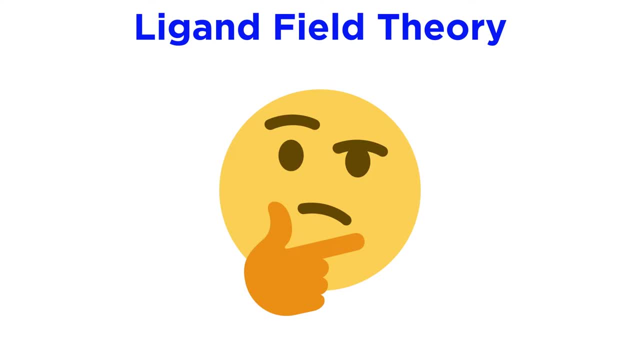 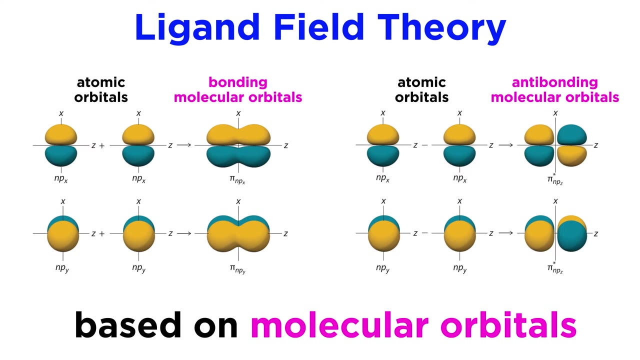 energy. Now we have to build on this understanding of bonding in transition metal complexes by supplementing with another theory called ligand field theory, which can be thought of as somewhat of an extension of crystal field theory. Ligand field theory is based on molecular orbital theory. 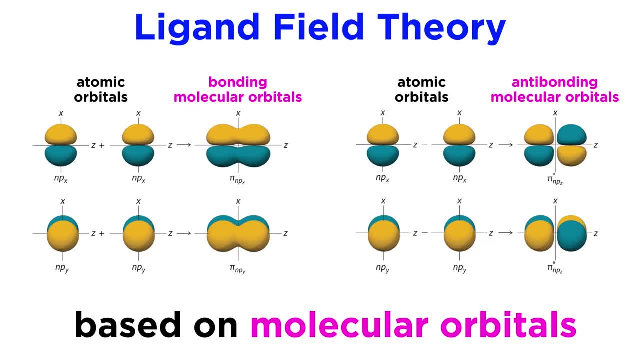 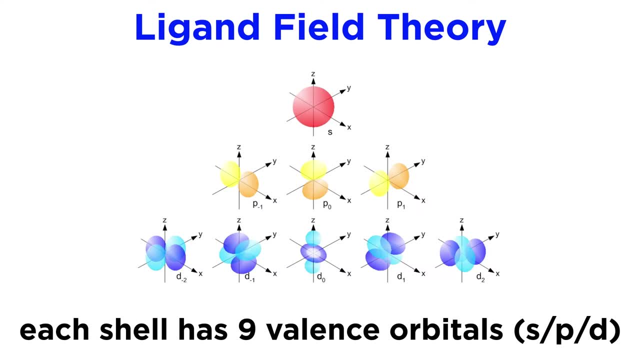 and it is a bit more successful in predicting certain properties of transition metal complexes, such as certain data gathered from spectral analysis. This model deals with the s, p and d orbitals that are possessed by a metal for a given shell, which gives a total of nine valence orbitals. 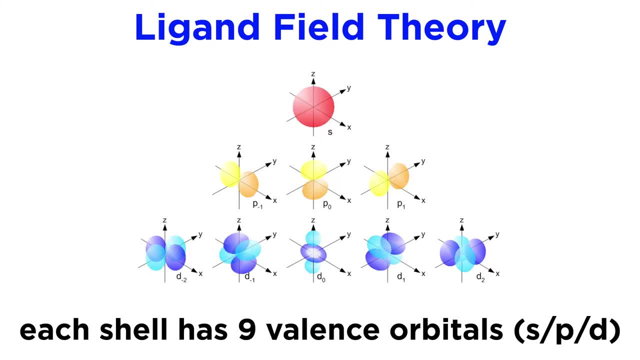 for the metal. The s, p and d orbitals that are possessed by a metal for a given shell, which gives a total of nine valence orbitals for the metal. The s and d orbitals that are possessed by a metal for a given shell, which gives a total of nine valence orbitals for the metal. The. 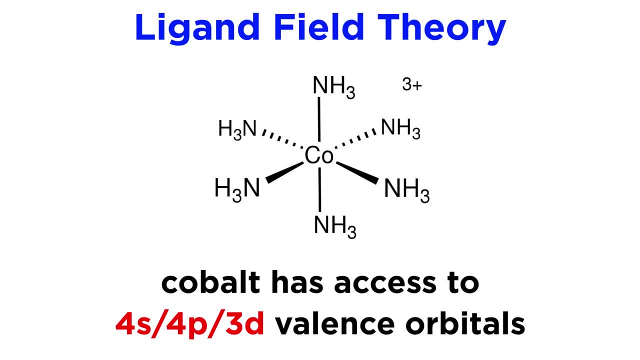 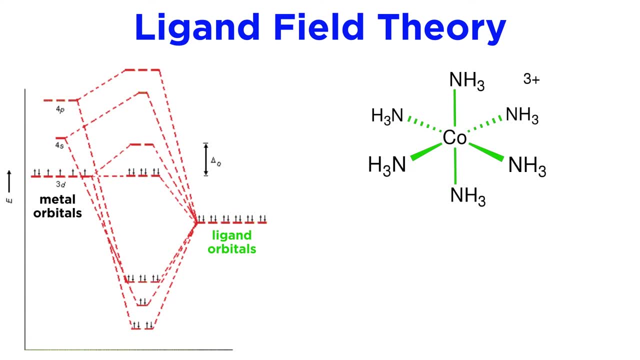 s, p and d orbitals that are possessed by a metal for a given shell, which gives a total of nine valence orbitals. for the metal, The S-orbical percent will be produced. Six of these are bonding orbitals, which are all of a lower energy than 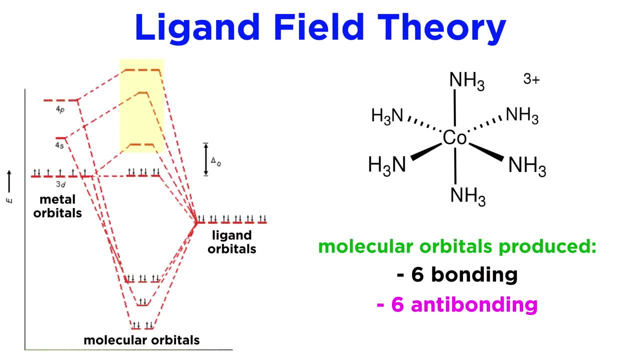 the original atomic orbitals. six are antibonding, which are of a higher energy than the original atomic orbitals, and the remaining three are non-bonding orbitals, which have the same energy as the 3D orbitals on the metal. The molecular orbitals are populated precisely as we would. 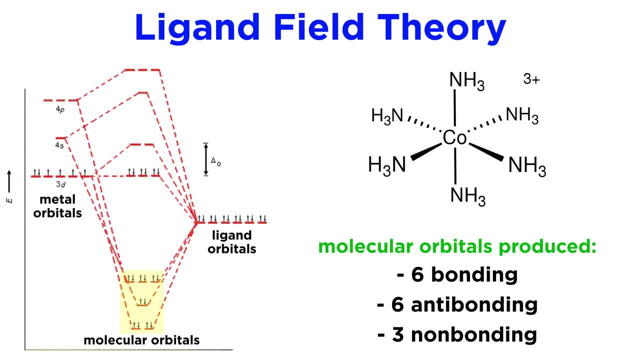 expect from lowest energy and moving upwards, which in this case leaves us with all of the bonding orbitals full, as well as the non-bonding and the antibonding are all empty. This results in a very stable octahedral complex where metal ligand bonding occurs due to the overlap of these. 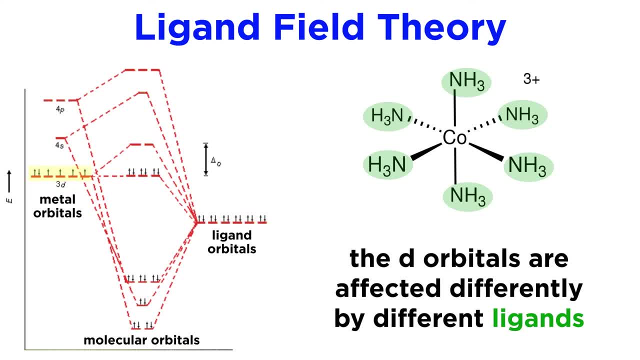 atomic orbitals, which accounts for covalent bonding Ligand field theory also describes the manner in which these d-orbitals are affected differently by different sets of ligands and can have their energies raised or lowered depending on the strength of their interaction with the ligands. 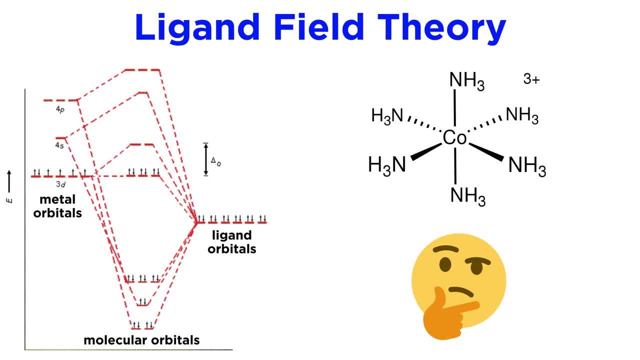 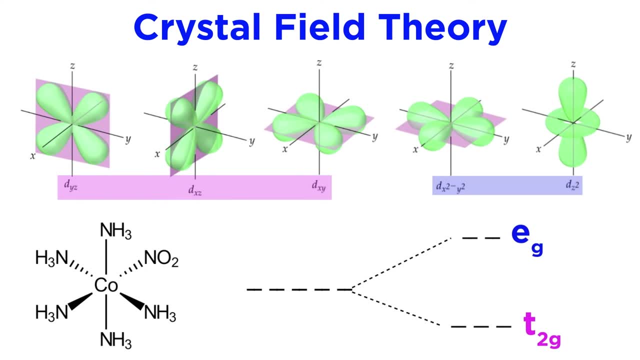 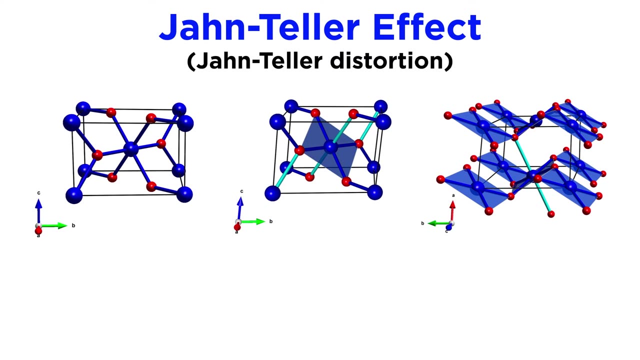 There is much more that we could discuss regarding ligand field theory, but let's return to crystal field theory and discuss a particular ramification that will be of interest to us in learning about transition metal complexes: The Jahn-Teller effect, also known as Jahn-Teller distortion. 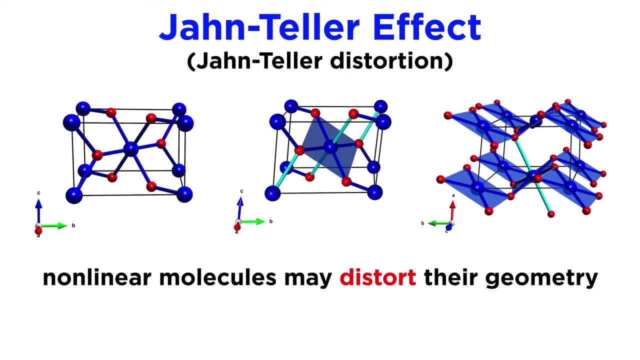 is a phenomenon which describes the way that non-linear molecules and, in particular, transition metal complexes, may distort their geometry in order to remove the degeneracy of unequal energy. This is a phenomenon that is often used to describe the way that non-linear molecules and, in particular, transition metal complexes, may distort their geometry in order to remove the degeneracy of unequal energy. 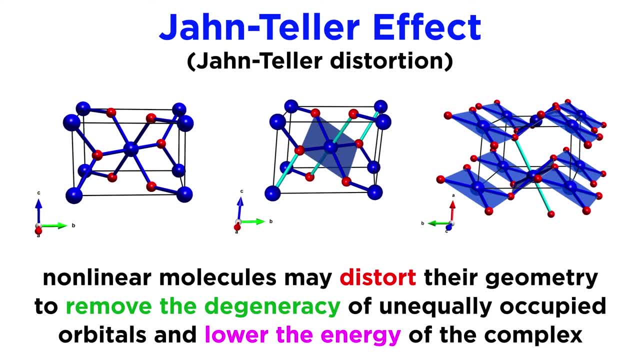 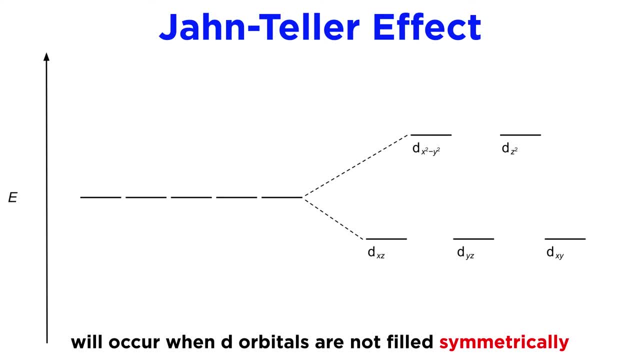 In other words, this is something that will happen when the d-orbitals are not filled in a symmetrical manner. Taking a typical octahedral complex, we recall that the d-orbitals are split up into the lower-energy T2G orbitals and the higher-energy EG orbitals, If electrons are arranged. 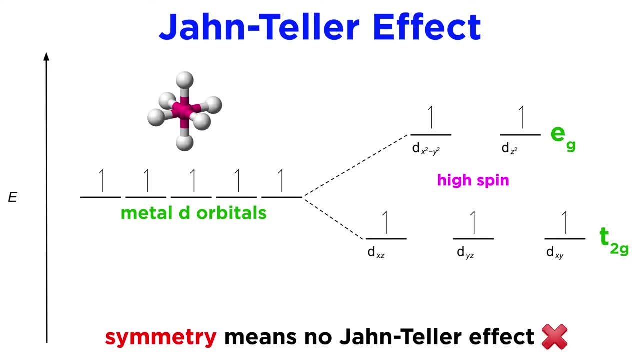 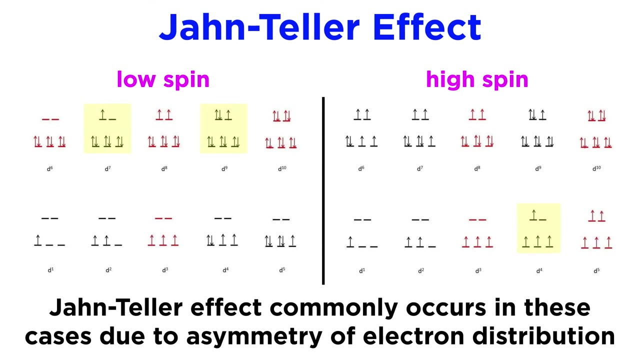 in these orbitals in a symmetrical manner. with one or both of these sets of orbitals either half-full or complete, the Jahn-Teller effect will not be observed In any other case it will. So high spin- d4, low spin- d7 or d9, these will be common situations that elicit the Jahn-Teller effect. 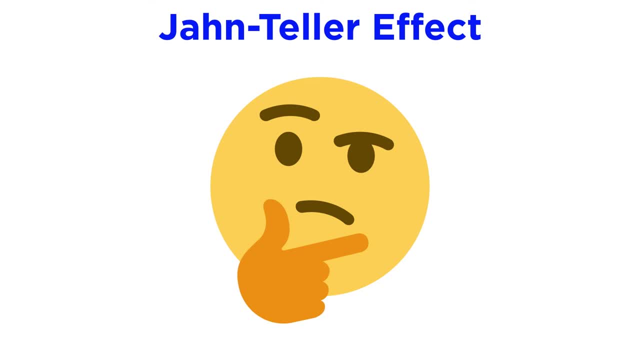 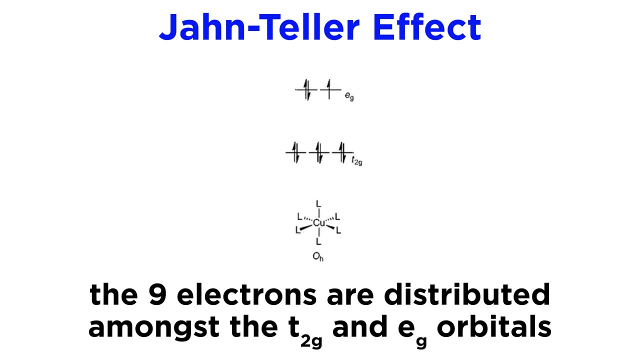 Let us now understand precisely what kind of distortion will occur. Take, for example, an octahedral copper complex with a two-plus charge. This will have nine electrons distributed around these d-orbitals, with the T2G orbitals completely full, while the EG orbitals 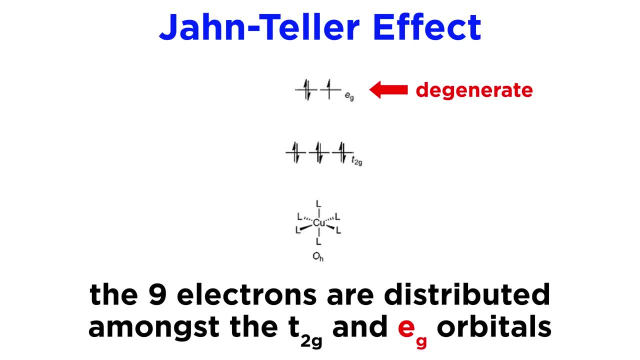 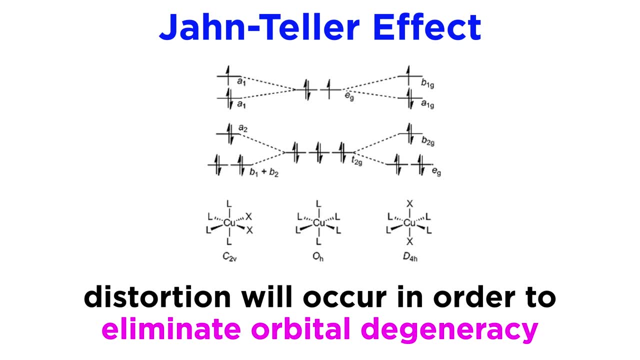 will be one full and the other half-full. These EG orbitals are degenerate, as shown, but the Jahn-Teller effect predicts that the complex will distort in such a way that the degeneracy is eliminated, which we call tetragonal distortion. When this happens between the dx-squared minus y-squared, 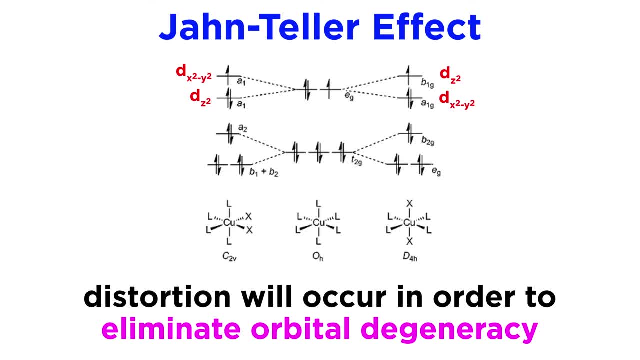 and dz-squared orbitals, one will become higher-energy t2g And they will end up the same distance away from the original orbital in energy in either direction. The same goes for the other three orbitals where the dxy will no longer be. 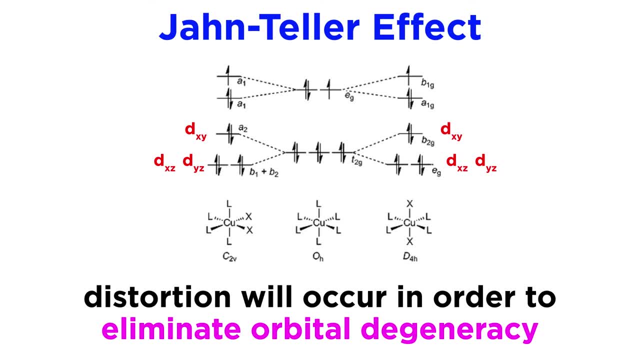 the same energy as the dxz and dyz. One set will be higher energy and the other set will be lower energy compared with the original energies, and the distance to the dxy will be twice the distance to the others because of the one-to-two ratio. As a result of this activity, the complex 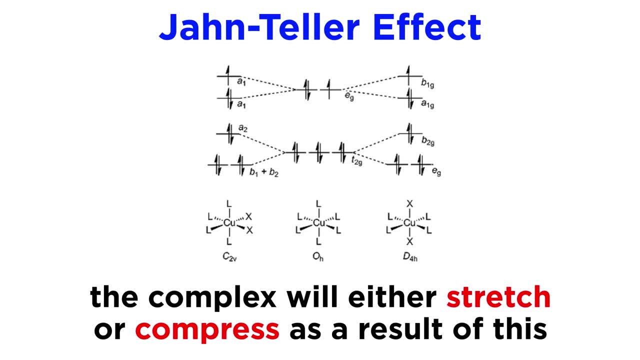 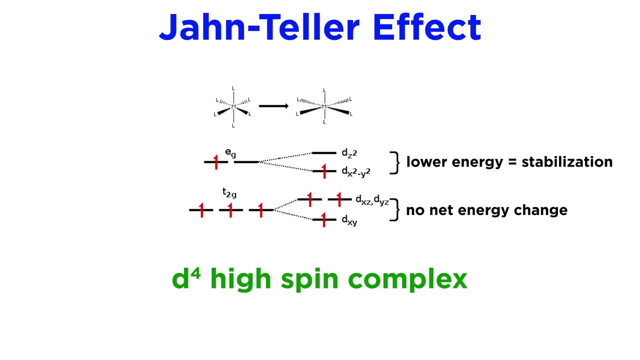 will either stretch or compress along the z-axis. If the asymmetry is in the T2G orbitals, the effect is weak. If in the EG orbitals, the effect is strong. Here are some examples so we can get a better understanding. First, a d4 high spin complex. 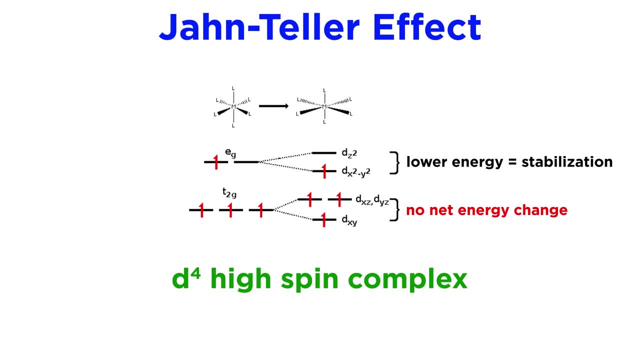 For these orbitals down here there is no net energy change. But for the ones up here this lone electron will become lower in energy as it moves to the dx-squared minus y-squared orbital. This stabilization produces a tetragonal compression, so the metal ligand bonds along the 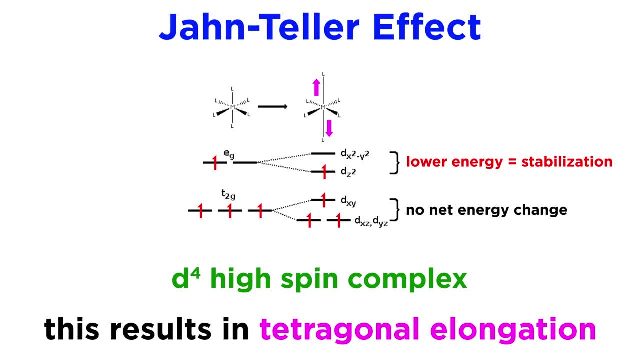 z-axis will compress. If, instead, the dz-squared orbital is the lower energy orbital for a d4 high spin complex, we will get the same stabilization, but we will observe tetragonal elongation, where these bonds will stretch instead of compress due to the shape and orientation of the dz-squared. 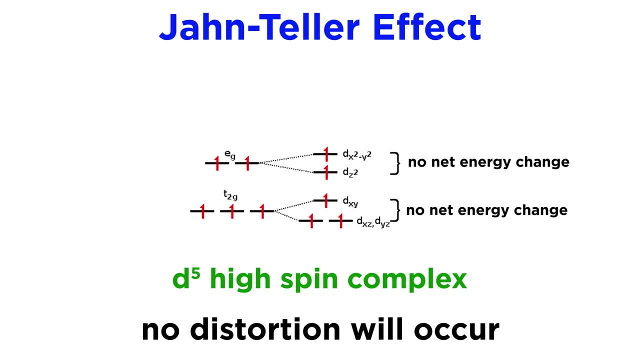 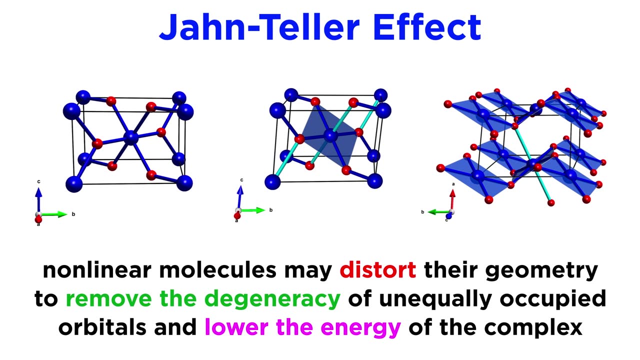 orbital, a D5 high spin complex, where now all the orbitals are half full. so when distributed amongst the new orbitals there is actually no net energy change and therefore no distortion. The Jahn-Teller effect will be something to keep in mind when considering the geometry. 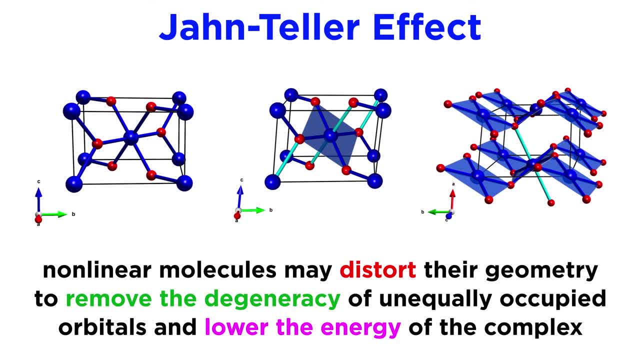 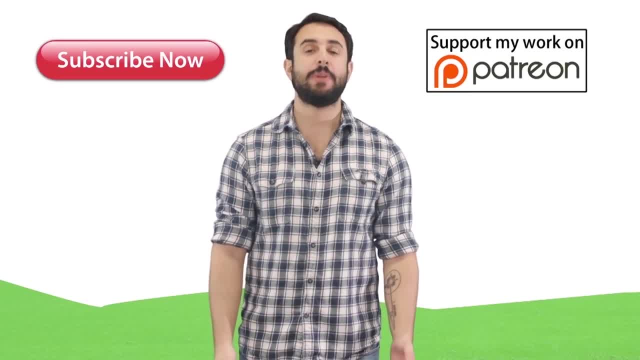 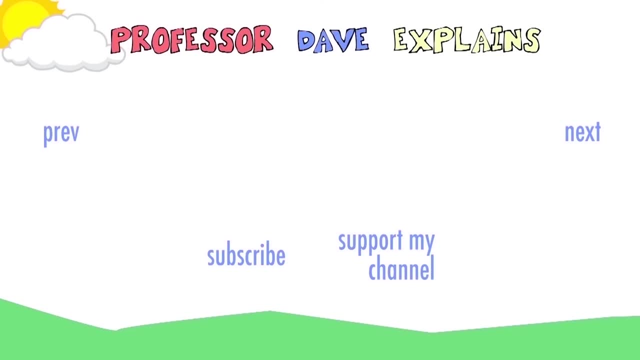 and properties of transition metal complexes. Now let's move on to our next topic in the series. Subtitles by the Amaraorg community.